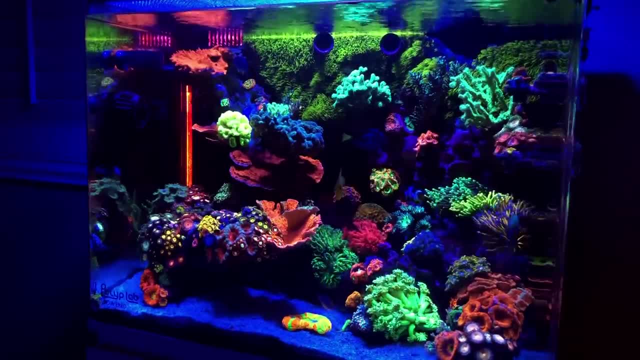 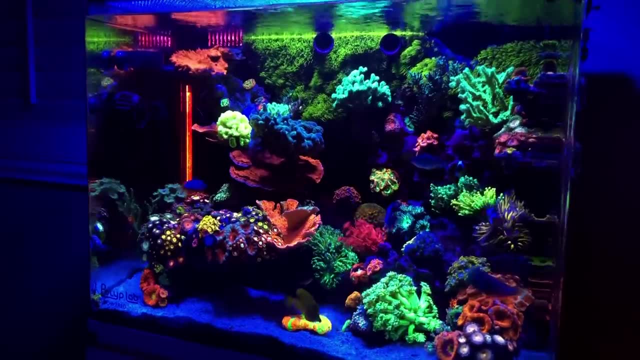 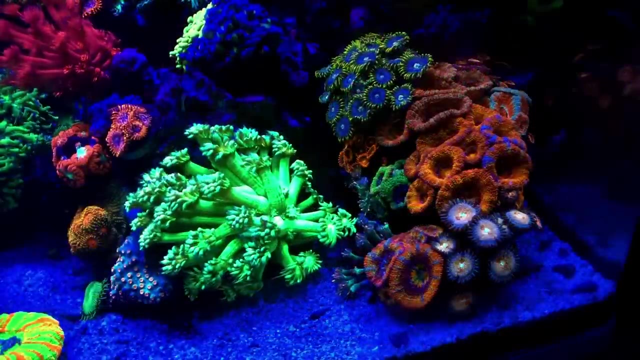 throughout my time here in the hobby. So one of the very first things I do want to talk about, because I get asked quite a bit, is number one: what lights do you run? So first of all, guys, I am running, as you guys can see here, two XR15 generation four lights. For you guys that have 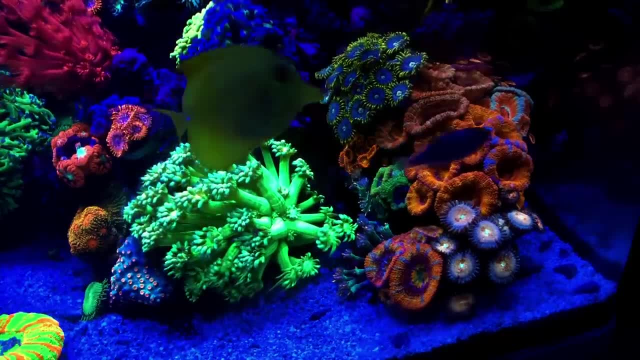 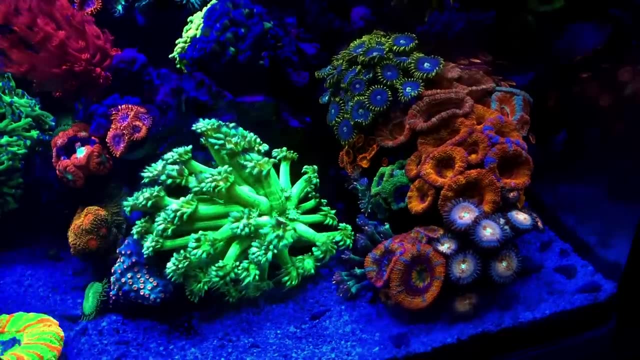 followed me for any length of time, you've probably seen that I used to have an XR30, and you're probably saying so. why the heck did you get rid of the XR30 and go with two 15s? Oh, but there's kind of a few reasons. My tank, specifically, is almost 30 inches wide. 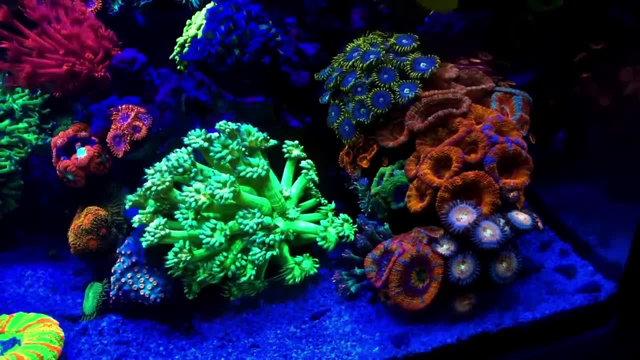 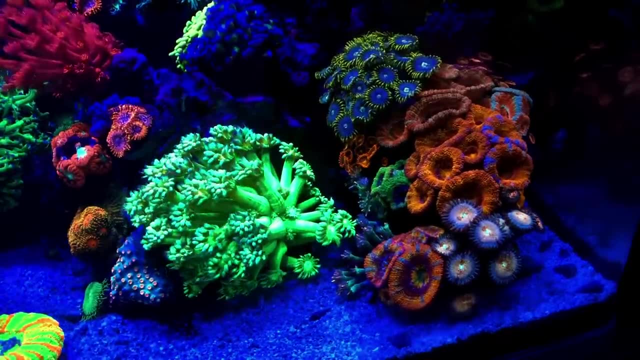 So when I had the 30 on there it was pretty good spread. but I noticed with the two 15s I was able to control the spread a lot better. You're probably saying, well, how do you do that? All you do is you really just open up the spacing a little bit and just gives you more control. 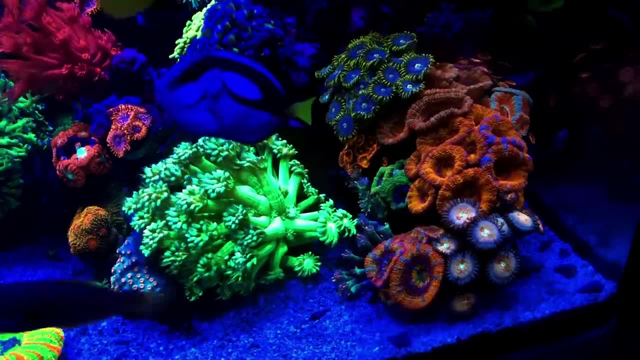 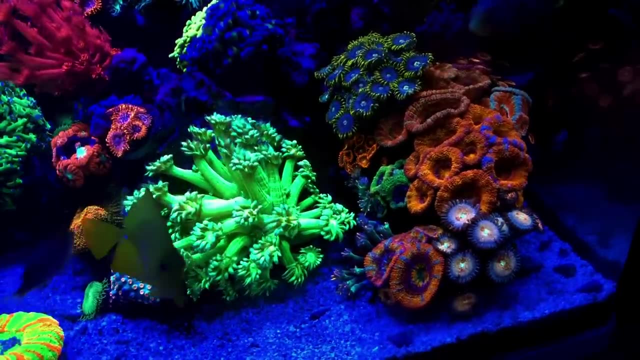 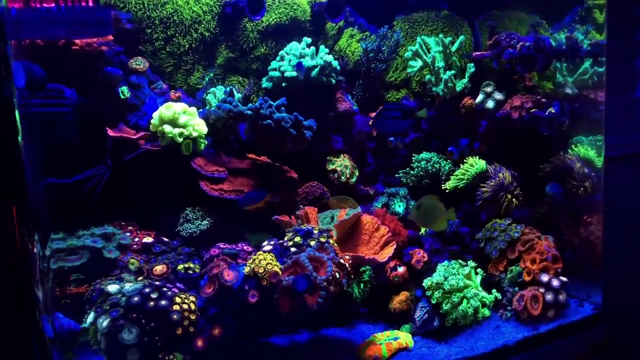 I'm obviously not going to keep this tank forever. I am going to go bigger. So that quickly opened up the gates to allow me to use both lights on a bigger tank without having to purchase any more lights. You know, if it was an XR30, there's really no way you can spread them apart, unless 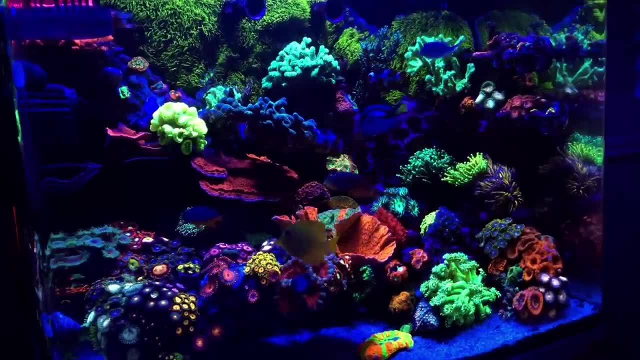 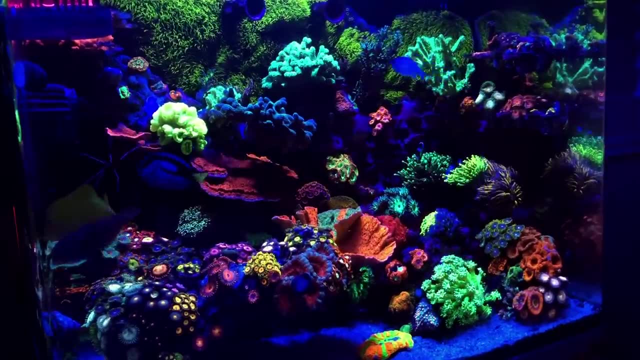 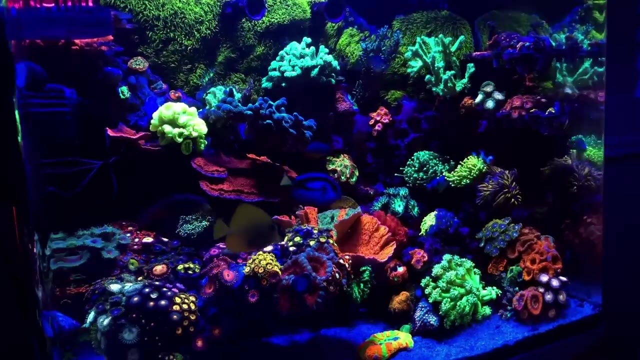 you cut the thing open and do a crazy DIY, which I would not be doing on a $800 light, But yeah, for upgradability. So that's also one of the main reasons I did the dual XR15, is one to have better spread And also for the upgradability. you know, if I do go with a 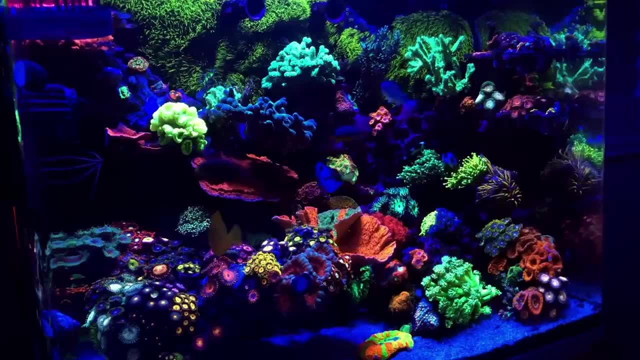 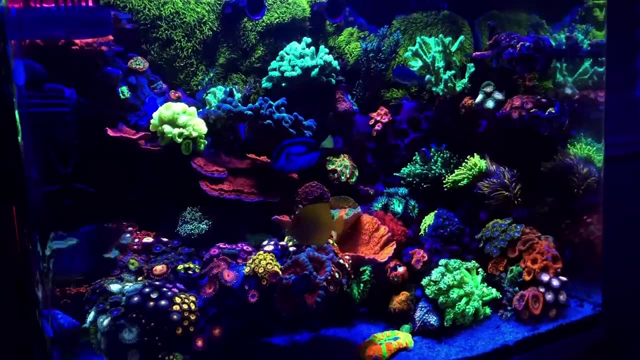 bigger tank. worst case scenario, I may have to buy one more at, you know, 400 bucks instead of 800 bucks. So that's kind of my take on that. I know a lot of people are always asking me: why did you do two 15s? Well, that's really the reason. As far as the power is concerned, 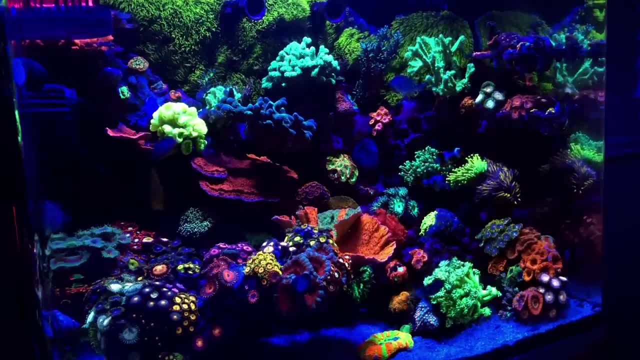 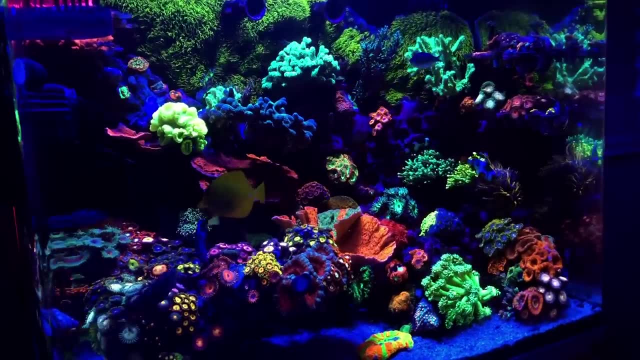 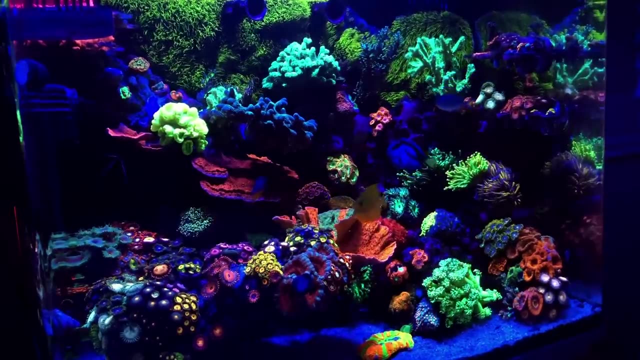 an XR15 is exactly half the power of an XR30.. It has the same LEDs on it, the same everything. So they're they're essentially the same exact light, just only one puck versus two. puck is really the only difference. So another thing: I get asked a lot. 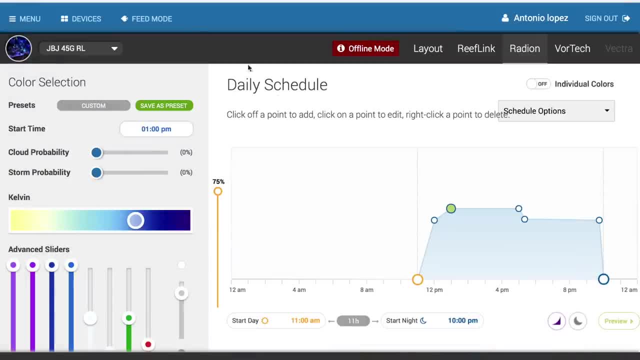 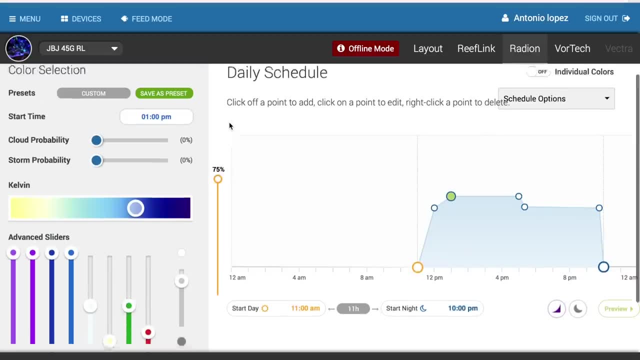 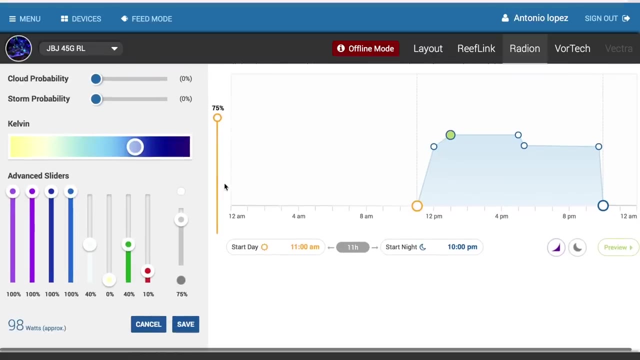 is of my light schedule. So I get asked quite a bit as far as my lighting schedule. So here you guys can see it: I'm running the light at an overall intensity of 75%. So just keep in mind this is 75%, assuming you put all the individual channels at 100%. 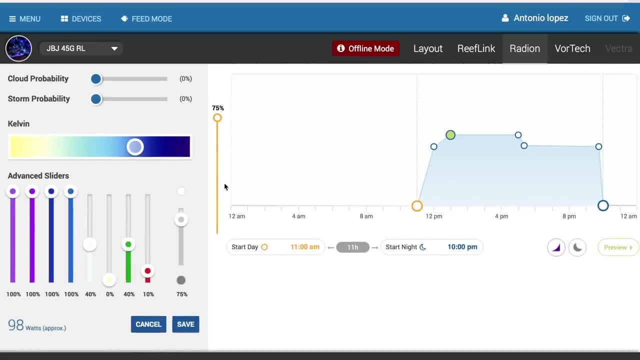 It's the maximum kind of they'll ever really go. So I am doing an 11 hour photo period kind of. starts at 11 in the morning from 10 at night. Typically I do this. I push it farther along the day because towards the mornings I'm not really at home, It just allows me to view the 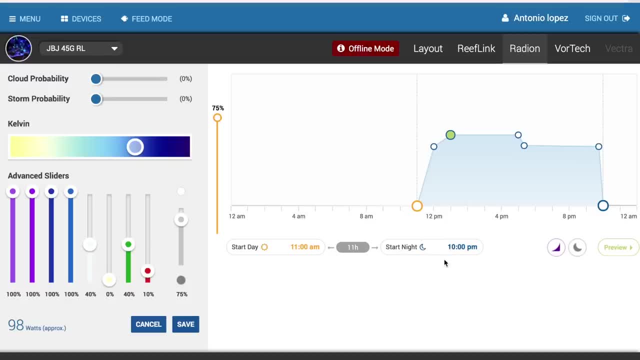 tank. you know, later on in the day, feed them, record them. you know what have you? So the program to tell you guys a little bit more about it, it's the same program Worldwide Corals uses Pretty much. it's a five hour white period and then five hour mainly blue period. given when I say 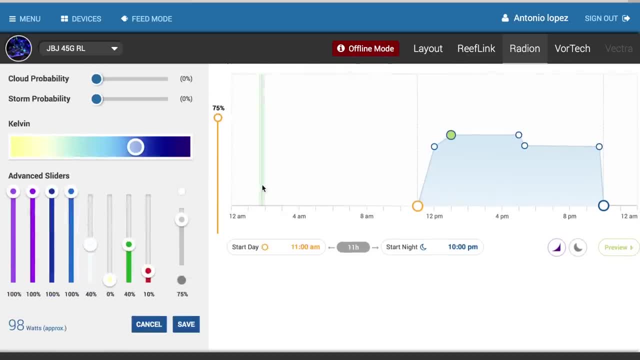 white, I don't mean 100% white. Here you can see the individual channels. So this is the first half of what I call the white period, with cool white at 40, warm white at zero, green at 40 and red at 10.. 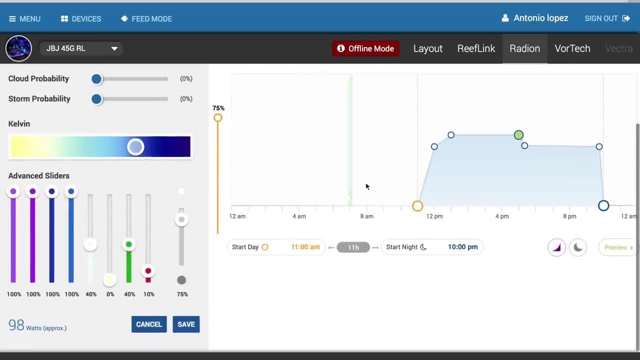 And that goes on till five. Again, it's the same same schedule, kind of a 520.. We ramp down to what I call a full blue, just with the hair of of a cool white, And this goes all the way on to 945. 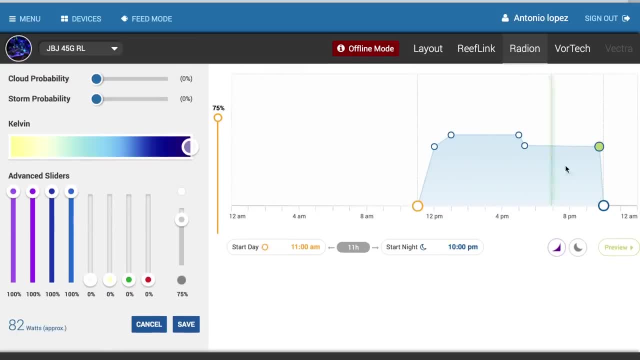 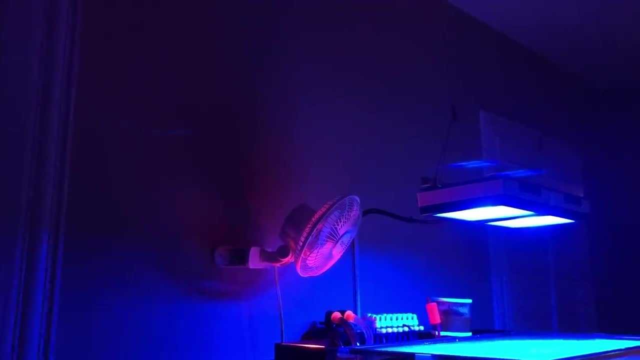 with the transition to full blues here and violets and then a 15 minute kind of just shut off from here. So now that we did get this, the my lighting schedule out of the way- hopefully answered a few questions there- I want to go a little bit more in depth on lighting, So this is going to be a little 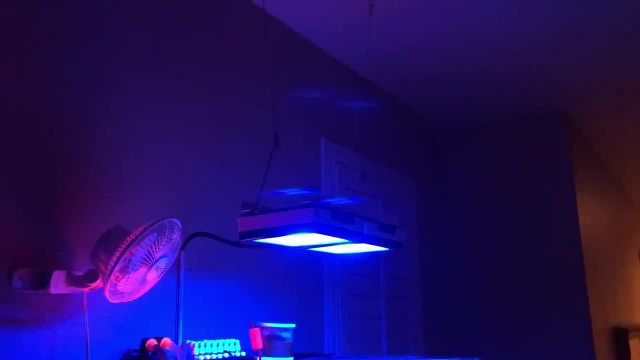 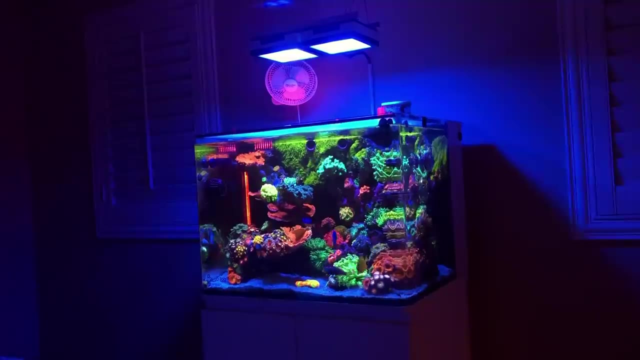 bit more geared towards intermediate, or intermediate and new reefers, And just in a little bit more. as far as lighting. so i think people tend to point way too quickly, quickly, the finger at lighting anytime there's an issue with a coral or corals. i can't even begin to tell you. 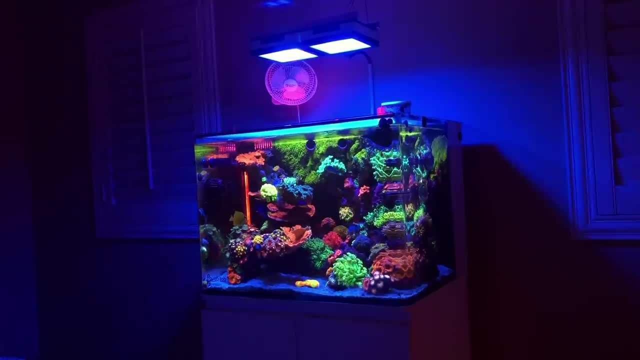 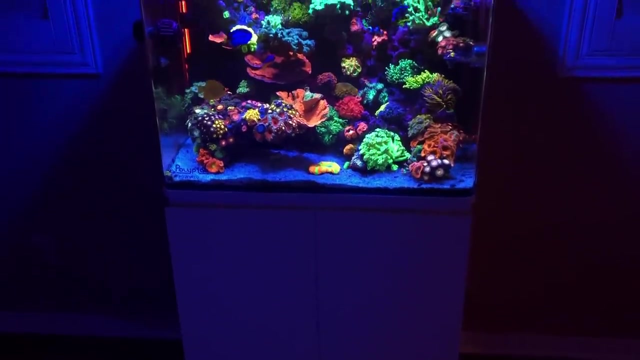 how many dms i get. you know, someone will send me something like: hey, my euphelia is an opening. should i add more blue? should i add more white? what should i do? and really, guys, almost 90 of the time lighting isn't to blame. it's a fluctuation in a parameter where i'm going with that stability. 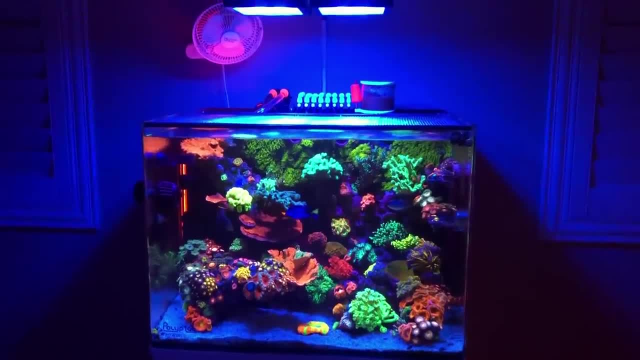 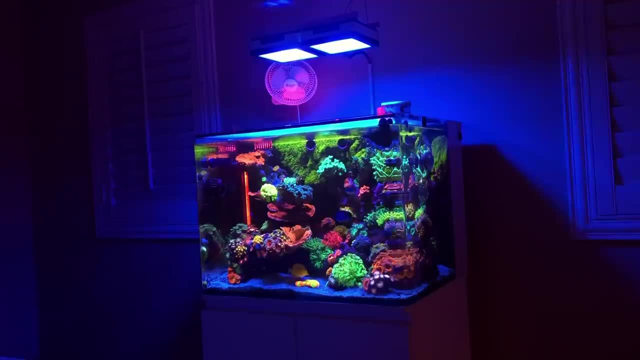 i think the first thing, anytime you see issues with the coral, you have to point the finger at some element, some trace elements, something in the water either fluctuating, changing and not staying consistent, thus stressing out the coral. i mean, there is cases when lighting can be an issue, but generally speaking, corals aren't that picky on how much. 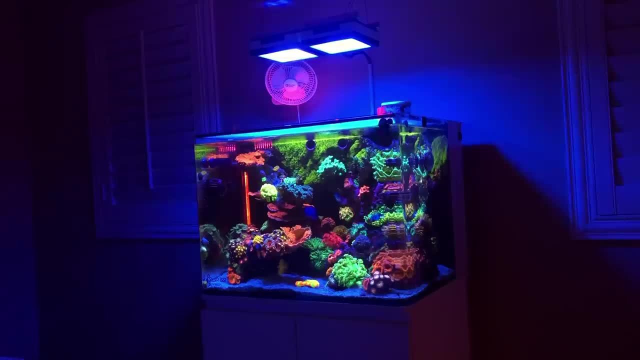 blue, how much white you're running? i mean given within reason, um, you know they'll, they'll take it pretty well. i see way too many people always logging on forums changing their template. you know, adding more blue, adding more white, and they do this on a regular basis. the thing you got to. realize, anytime you make a change to lighting, it's gonna, in essence, shock the coral and it's gonna take anywhere from one to two months for it to really get back on track and start growing really happy again. so just keep that in mind: that if you are going to do changes, it's going to take 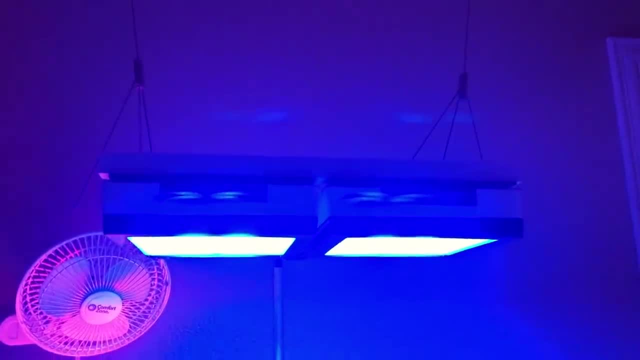 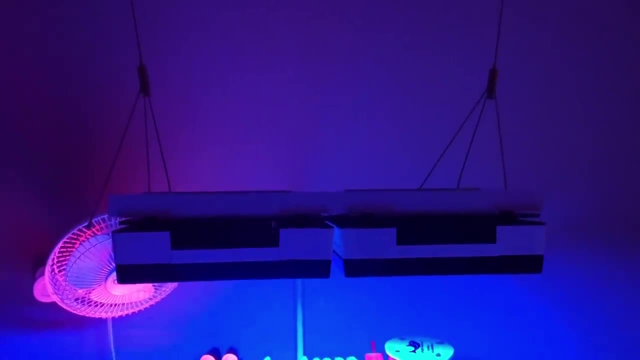 a while. for the coral to come back now for you guys watching. maybe you got your first set of lights and you're saying so what color should i run? generally speaking, the numbers i'm going to give you here are pretty good all across the board. doesn't really matter the brand of lighting, so a 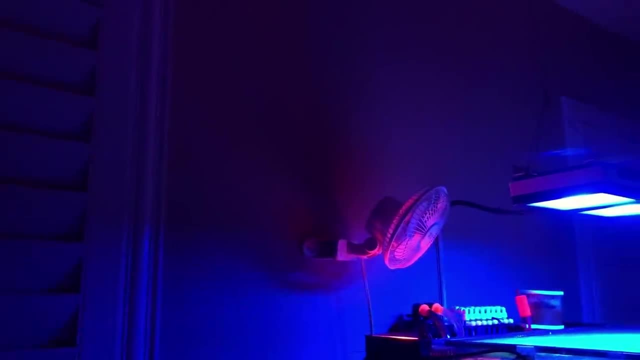 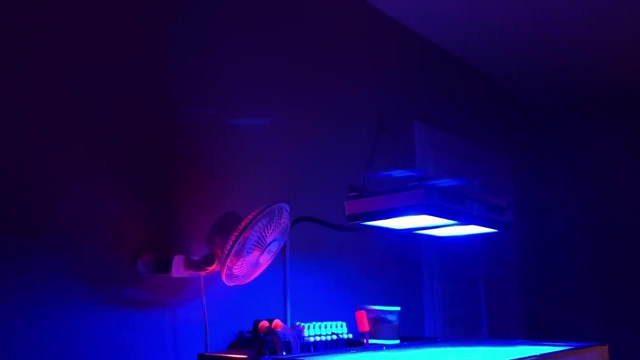 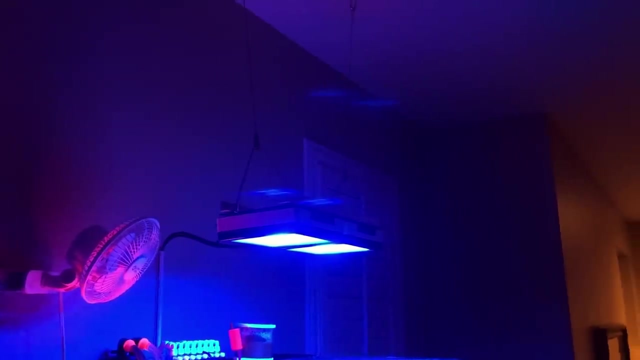 good schedule, good template. to start off with your violets and blues, put those at about 100 for your white channels to run those anywhere from five to thirty percent, depending on the look you're going for. as far as the green and red channels, try and keep those under 20 and you should be good to go again. 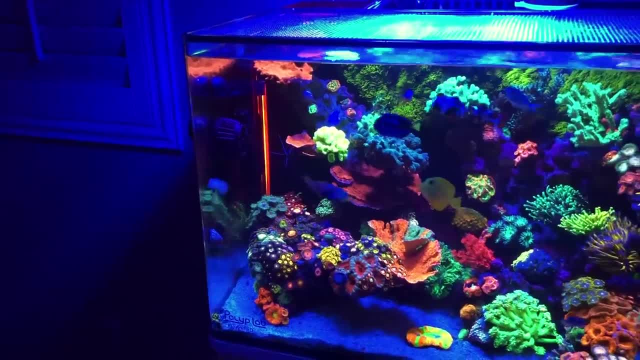 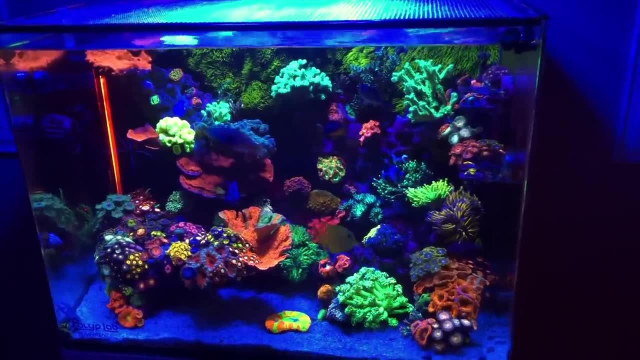 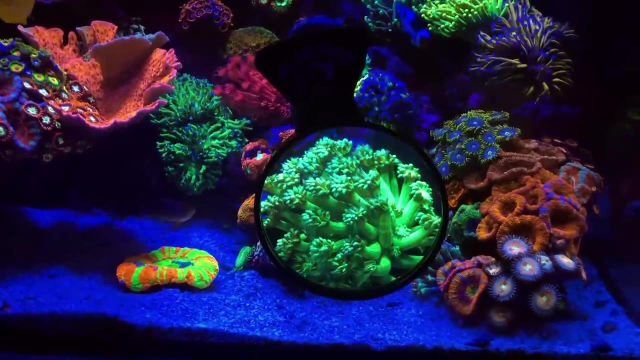 that's a good starting point, and don't be that person that's always trying to change the schedule because john told you, because bob told you. um, you know, the main thing and the main reason why reef tanks do well and corals thrive is because is because stability. you know? yes, it's a. 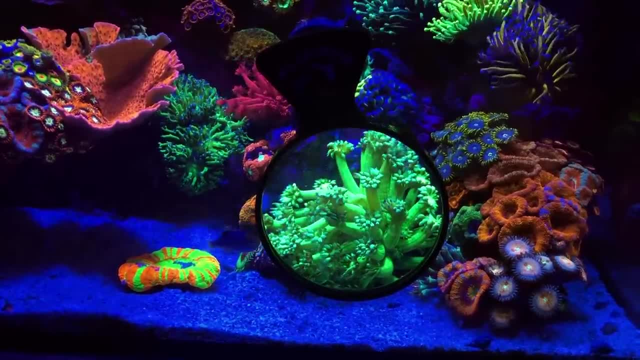 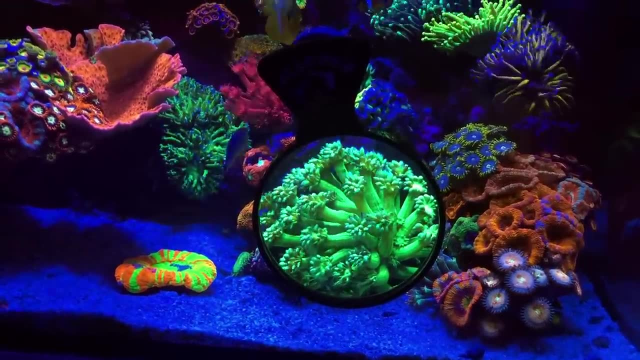 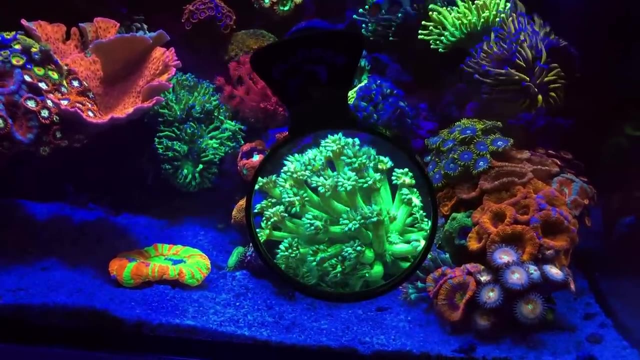 little bit to do with the lighting, um, but more you know, in more cases than not, it's the stability in the water. so you know. from this point forward, i guess, if you have an issue, have lighting be one of the last things you look at and one of the last things you adjust, because you can't imagine how. 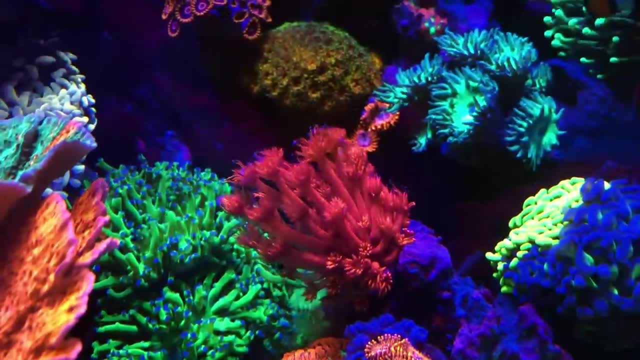 many people send me messages. you know a coral will be acting up and they'll change the lighting, and they'll do it on and on and on. so that's also kind of the reason why t5, the boll읍ie gulf test approach- was really interesting, because t5 is really great for 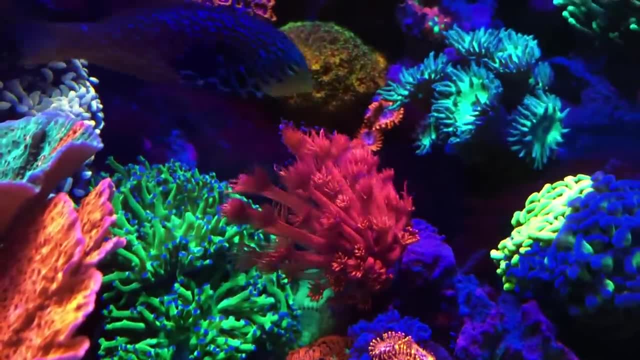 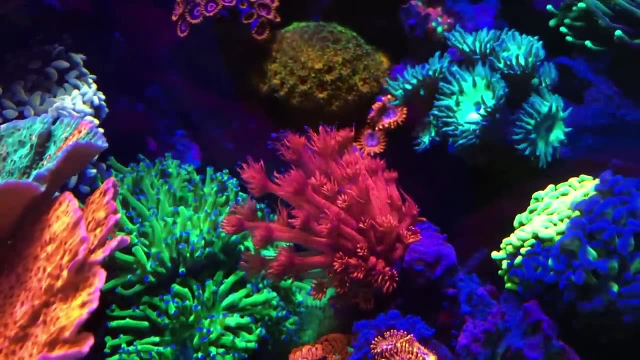 when you wanted to see your followers doing things like around the world and you're looking for, you know, is such a great uh light it's. it's really non-adjustable. it's either on or off and it's pretty much done. there's no way you can adjust it. that's one of the reasons why so many people. 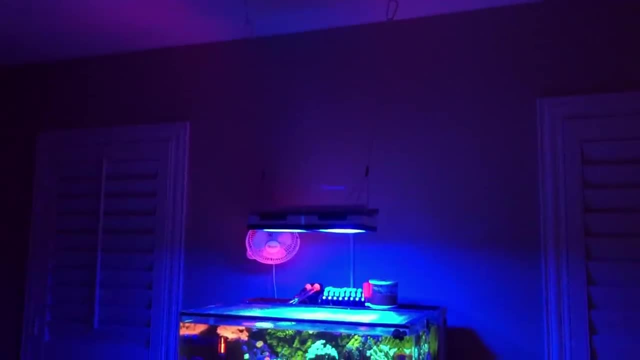 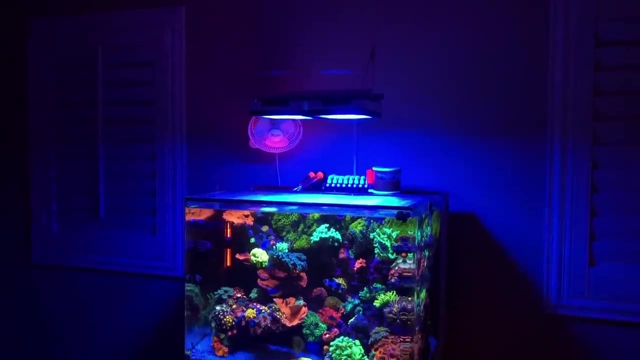 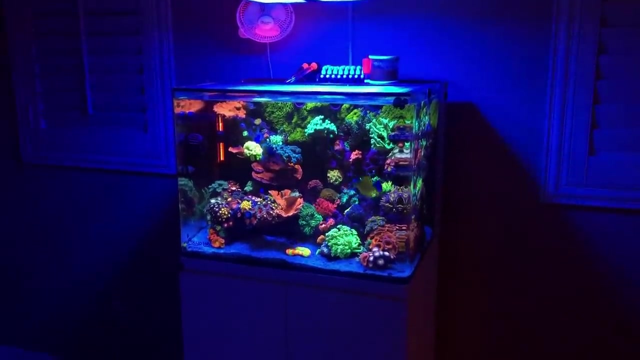 have had success with t5, now with led lighting. i mean it's good they're so customizable, but at the same time that's kind of one of the downfalls- not of the light, more of the user, because we're just always trying to tinker. i mean i probably haven't adjusted my lights in months, months, months and 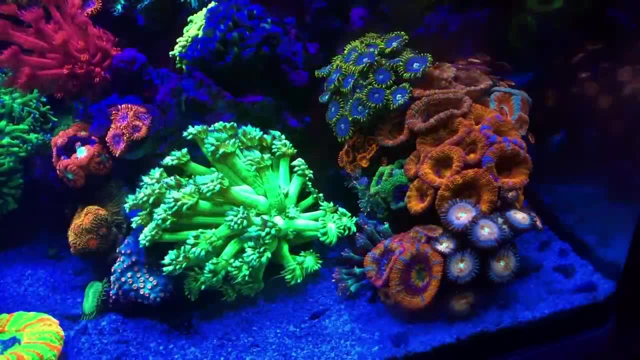 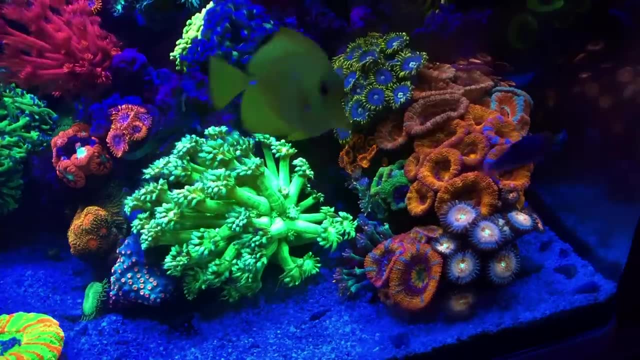 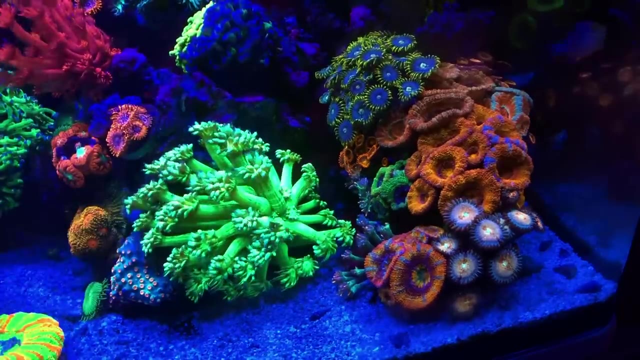 mainly when i do make adjustments. it's more on the intensity now and i do it over typically about six week acclimation. anytime i'm increasing the intensity, so hopefully i was able to shed some light. guys, i think people try to focus too much on lighting and just wanted to let you know. 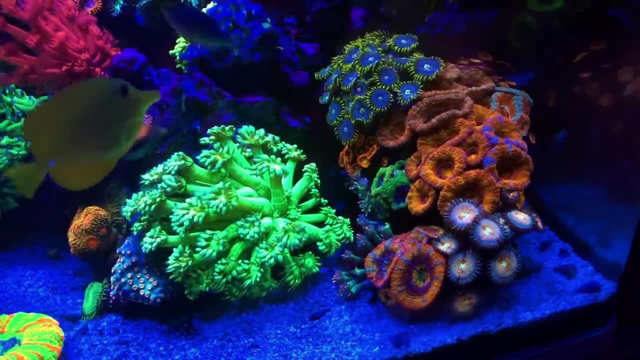 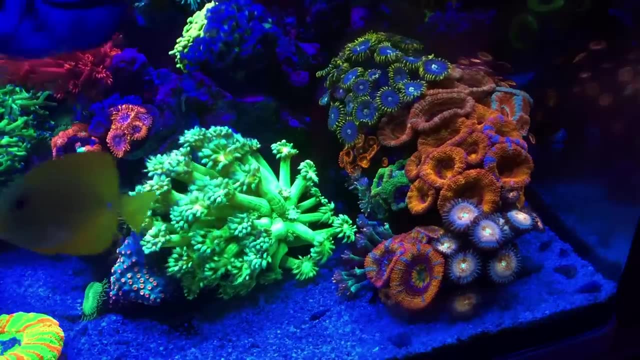 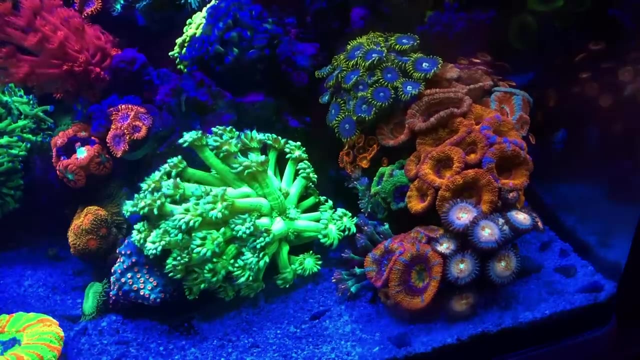 it's not, yes, it is important. i'm not trying to say it's not important, it's not as important as you think. um to hit that that specific uh spectrum. you know corals will accept quite a big broad of spectrum. so anytime you know you do run into an issue from 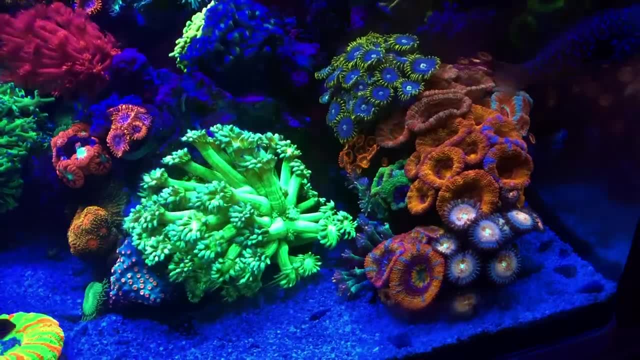 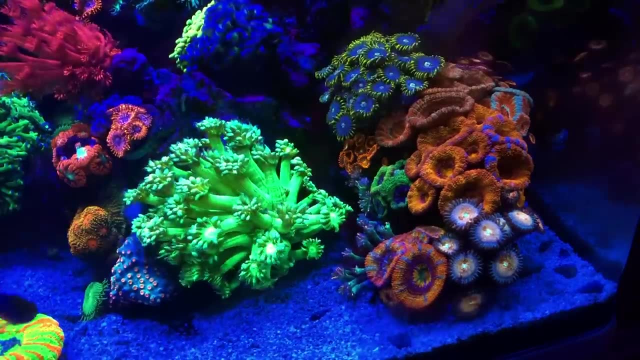 this point forward. you know, have lighting be one of the last things you check or last things you adjust. it's probably something else in your water column. uh, that's getting them pissed off, so we're gonna leave this video here. guys, i'd love to hear your experiences. what do you think about my? 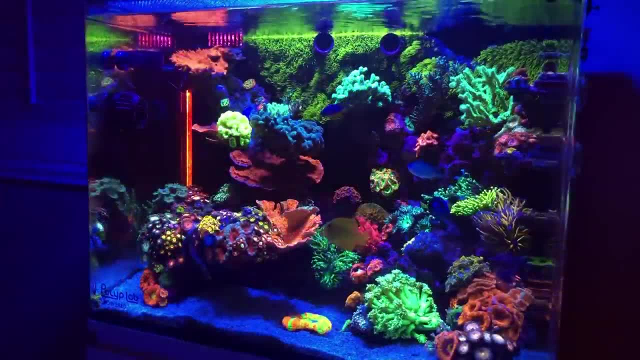 thoughts on lighting. do you feel as well as you do about it and i'll see you in the next video? all that, there's too many people trying to adjust them. i'd love to hear what you got to say down in the comment box below. so we're gonna leave this video here. guys, i want to thank each and every one. 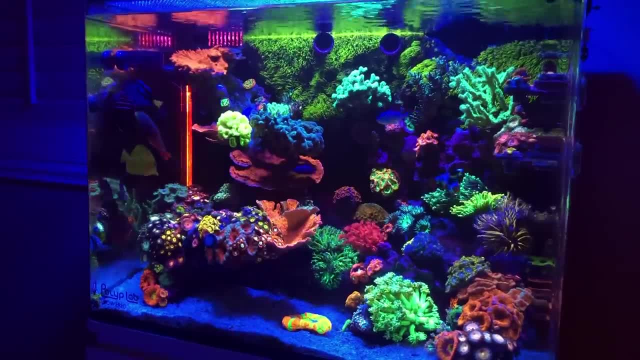 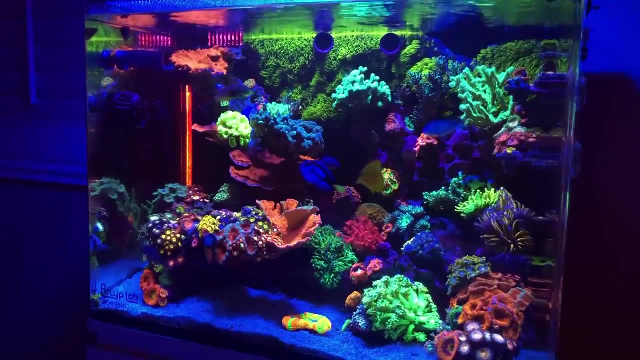 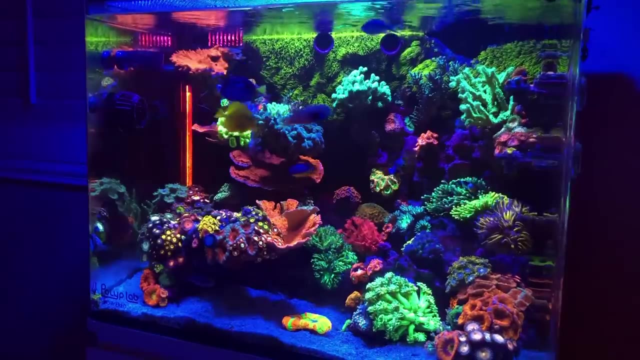 of you for helping me. that has subscribed. we just surpassed 7 000 subscribers here on youtube as well. on instagram. we're about to hit 20 000 followers. guys, i'm beyond blown away, so i want to thank each and every one of you. if you're watching and you're not subscribed here to my channel, maybe i earned.